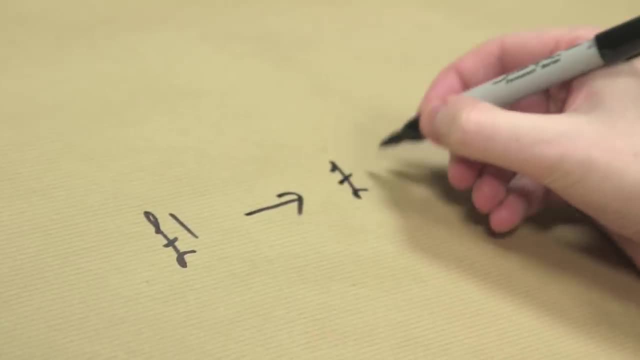 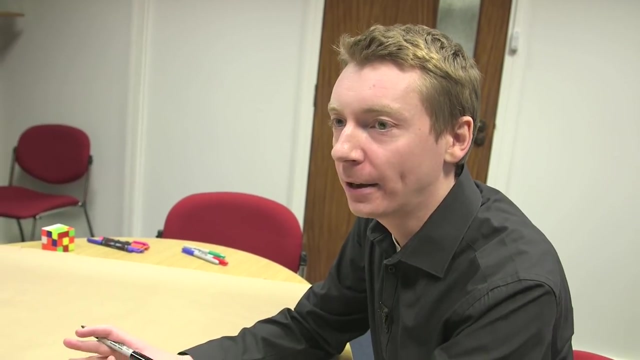 interest. so it means, after one year you'll have two pounds. So you've earned one pound interest and you've got your original pound. So you now have two pounds. What if I offered you instead 50% interest every six months Now? is that better or worse? 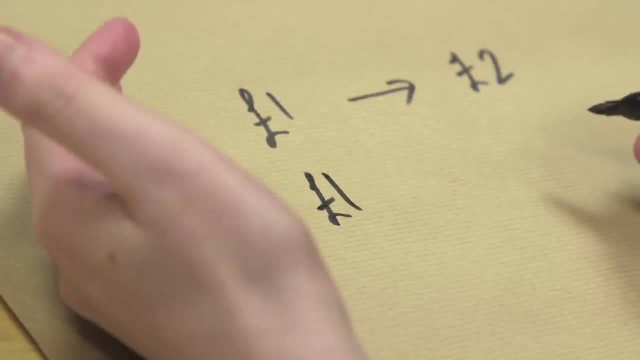 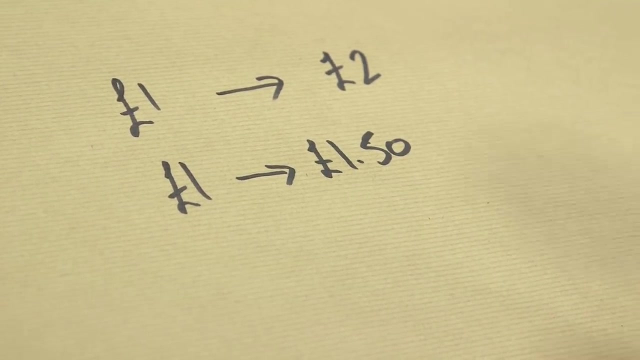 Smaller or worse. Well, let's think about it. OK, you're starting with one pound and then I'm going to offer you 50% interest every six months. So after six months you now have £1.50, and then you wait another six months and you're earning 50% interest on your total. 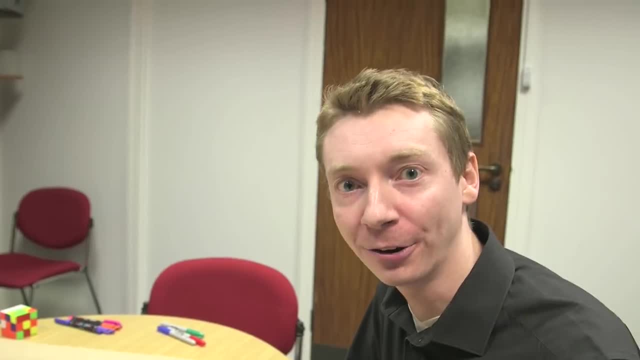 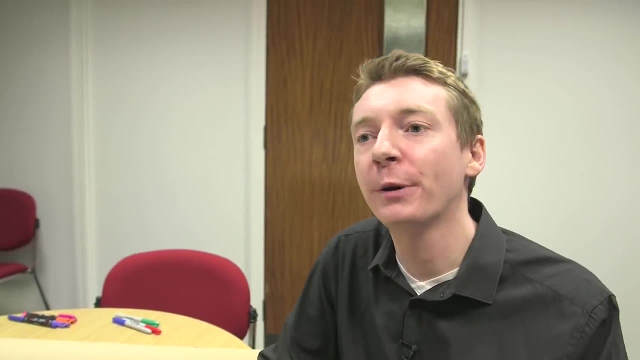 which is another 75p, And then you add that onto what you had, so it's £2.25.. So it's better, It's better. So what happens if I do this more regularly? What if I do it every month? I offer you one twelfth. 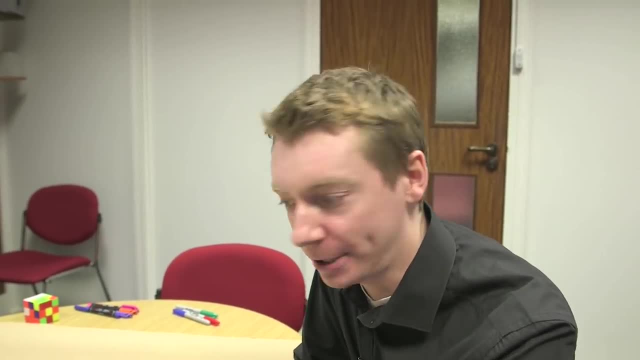 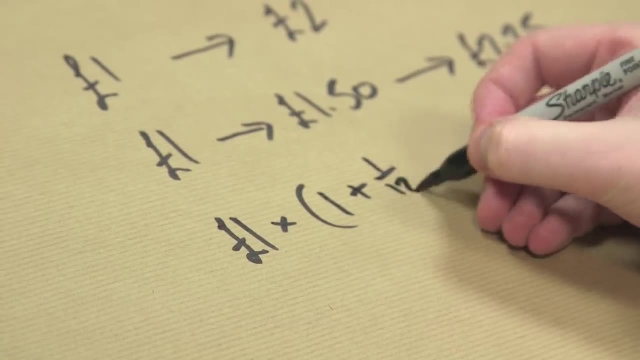 interest every every month. Is that better? So let's think about that. So after the first month, it's going to be multiplied by this, 1 plus 1 twelfth. So 1 twelfth, that's your interest, and then 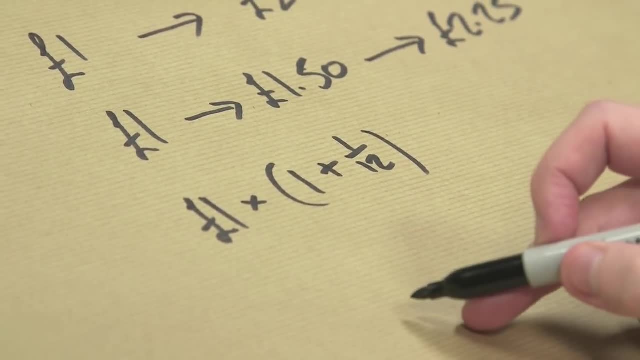 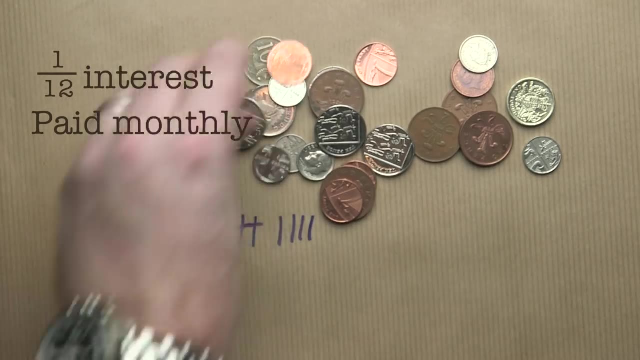 you're adding that onto the original pound that you've got. So you do that. that's your first month, And then for your second month you take that and multiply it again by the same value, And then your third month. you would multiply it again and again. You actually 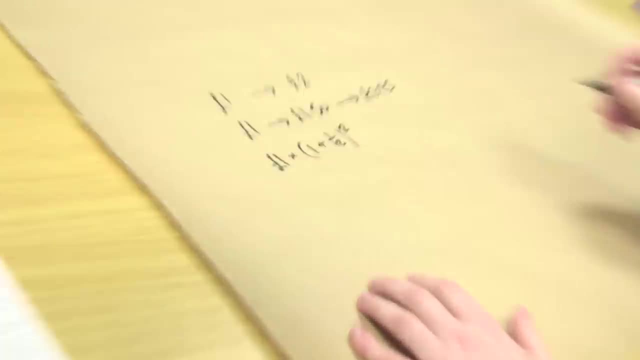 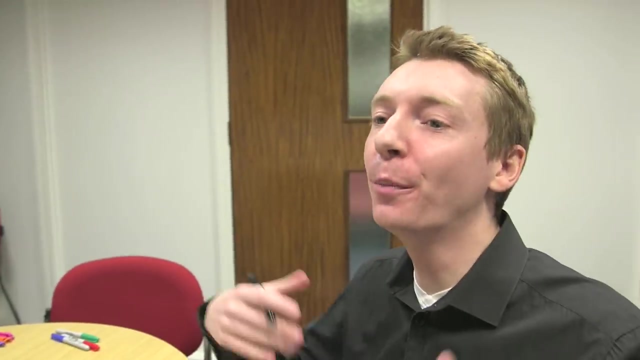 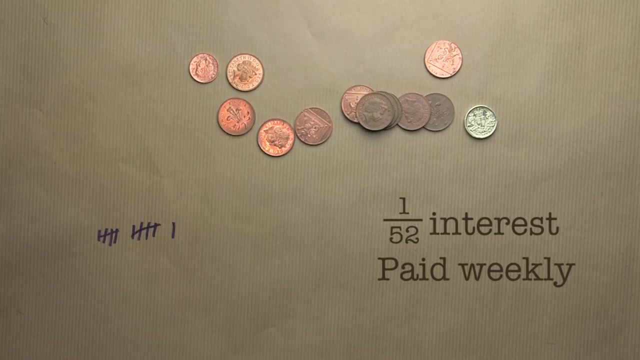 do that 12 times in a year. So in a year you would raise that to the power of 12, and you would get £2.61.. So it's actually better. In fact, the more frequent your interest is, the better the result. Let's start with every week. OK, so if we do it for every week, how? 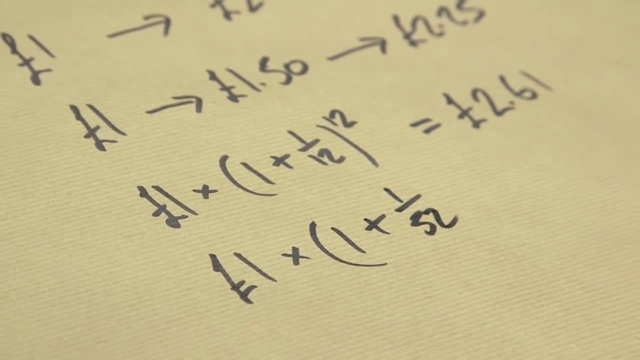 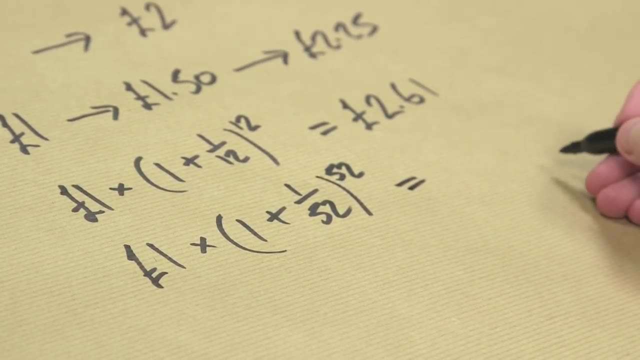 much better. is that OK? what I'm saying is you're earning 1 over 52 interest every week And then after the end of the year you've got 52 weeks and you would have £2.60.. So it's getting better and better and better In general. you might be able to see a pattern. 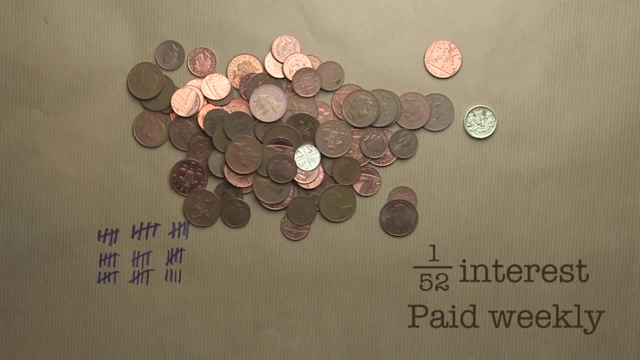 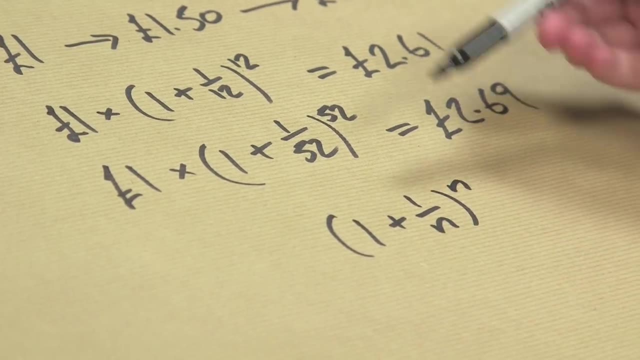 happening here. In general it would look like this: You'd be multiplying by 1 plus 1 over n to the power n. Hopefully you can see that pattern happening. So here: n is equal to 12 if you do it every month, 52 if you do it every week. If you did it every. 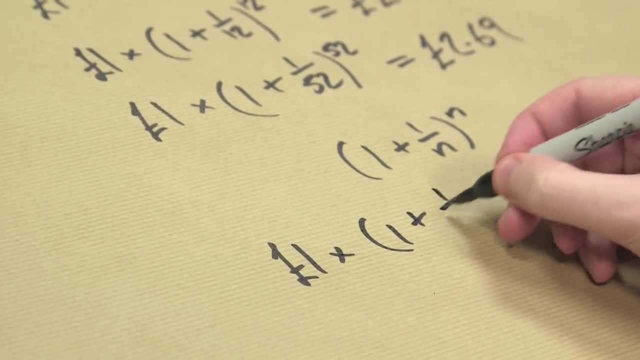 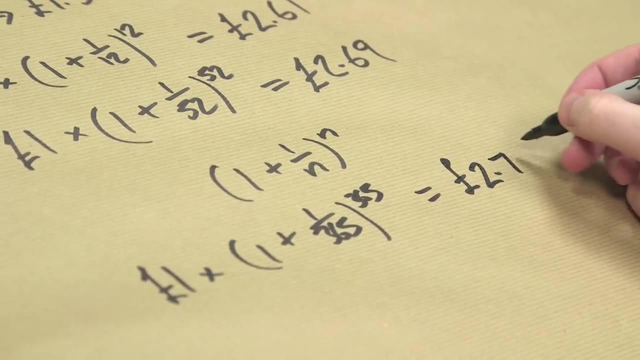 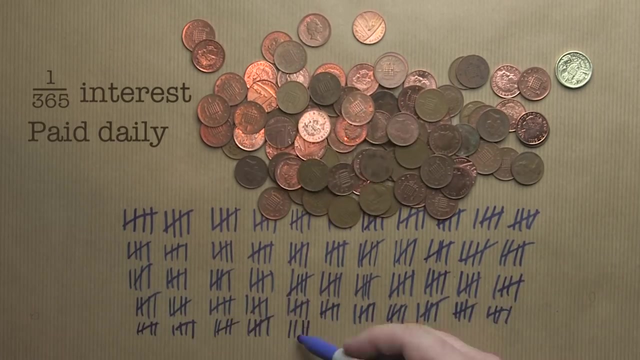 day. it'd be £1 multiplied by 1 over 365 to the power of 365. And that's equal to £2.71.. And so it would get better if you did it every second or every nanosecond. What if I could? 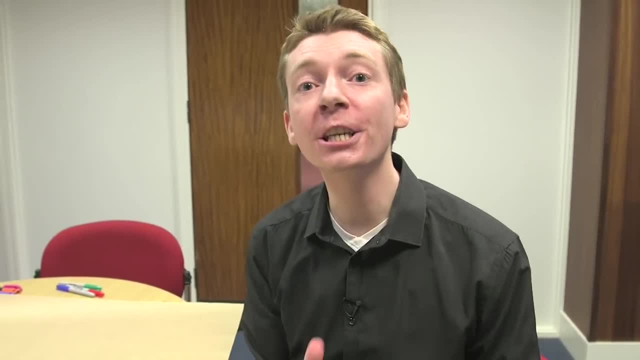 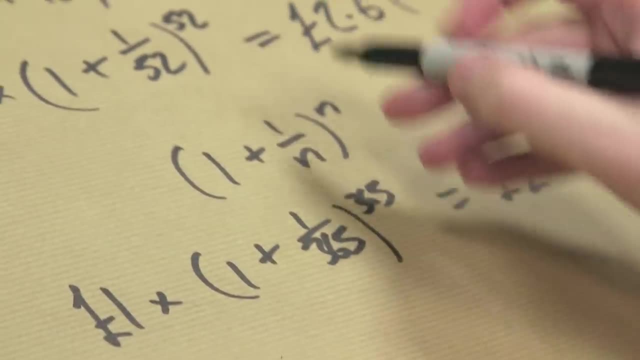 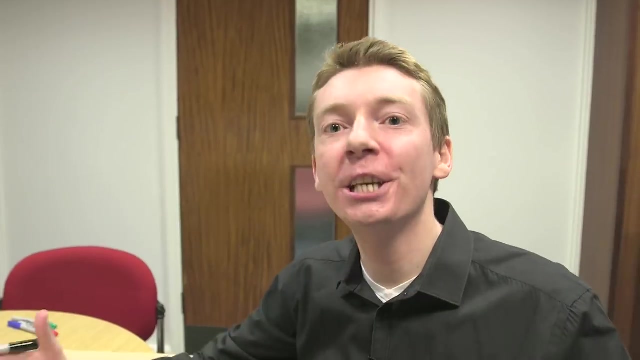 do it continuously. Every instant, I'm earning interest, continuous interest. What does that look like? That means, if I take this formula here: 1 plus 1 over n to the n, I'm going to n tend to infinity. That would be continuous interest. Now, what is that? What? 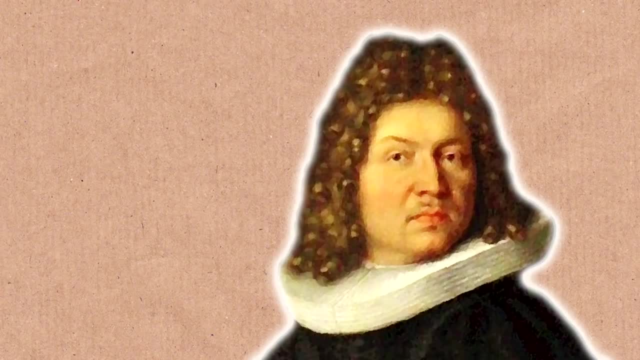 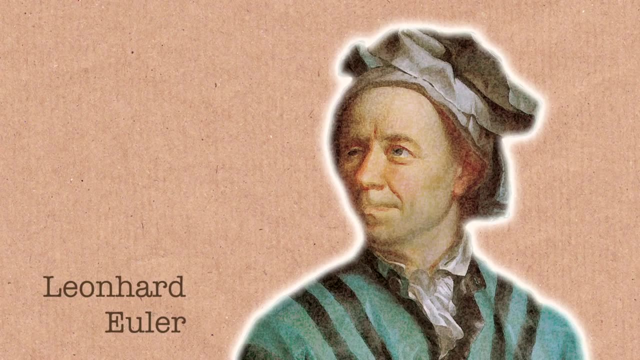 is that value? And that's what Bernoulli wanted to know. He didn't work it out. He knew it was between 2 and 3.. So 50 years later, Euler worked it out. Euler, he works everything out. 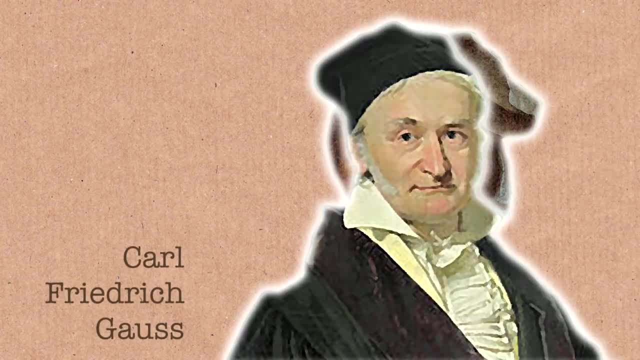 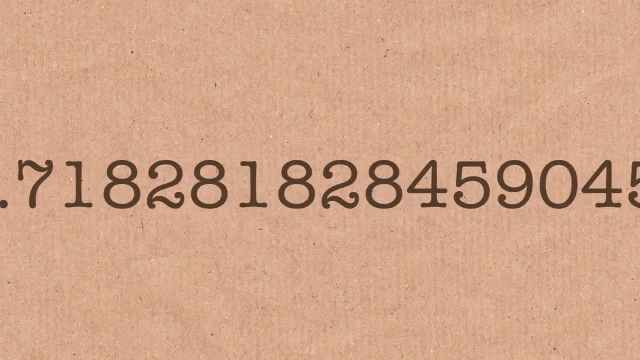 Anymore, Gauss. It's either Euler or Gauss. Say Euler or Gauss, you're probably going to be right. And the value was 2.718281828459 and so on. We were pretty close when we were doing it daily, weren't we? It was already 2.71 at. 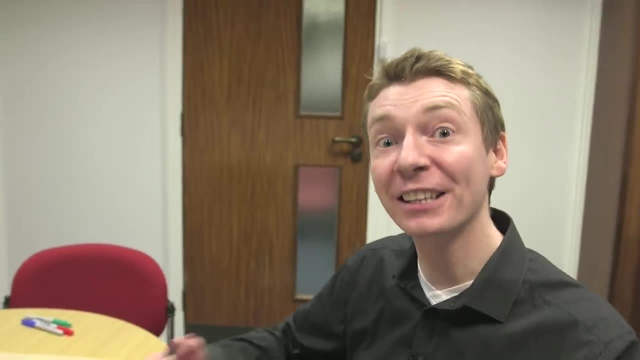 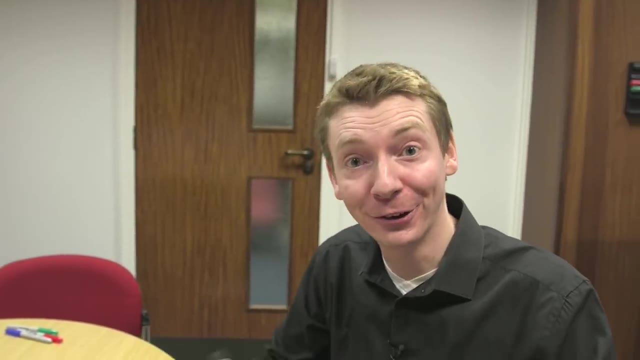 daily, You're right. You're right, We're getting closer, weren't we? We're getting closer and closer to this value, So already we're quite close to it. If you did it forever, though, of course you would have this irrational. 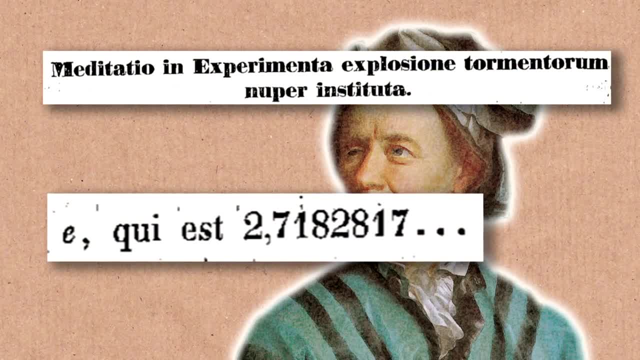 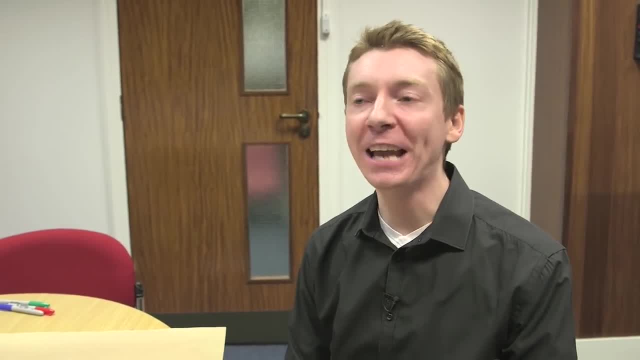 number. Now, Euler called this E. He didn't name it after himself, although it is now known as the Euler constant. Why did he call it E then It was just a letter. He might have used A, B, C and D already for something else, So 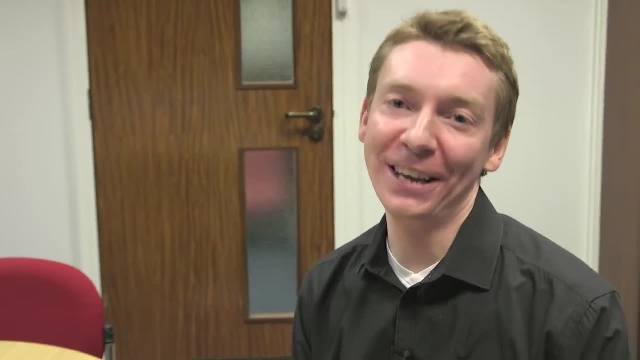 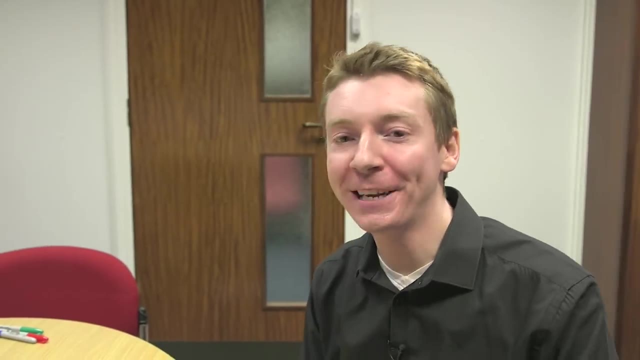 you use the next one. Bit of a coincidence. It's a lovely coincidence. I fully believe that he's not being a genius, He's not being a jerk here naming it after himself, But it's a lovely coincidence that it's E for. 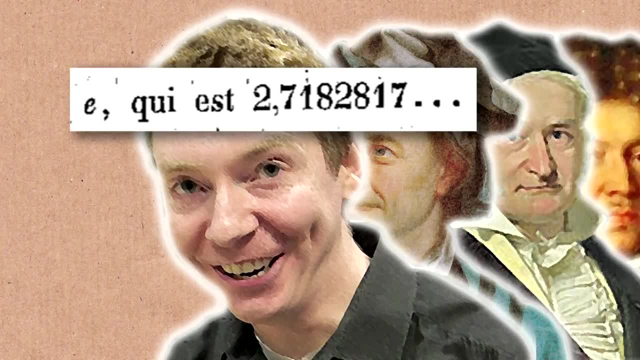 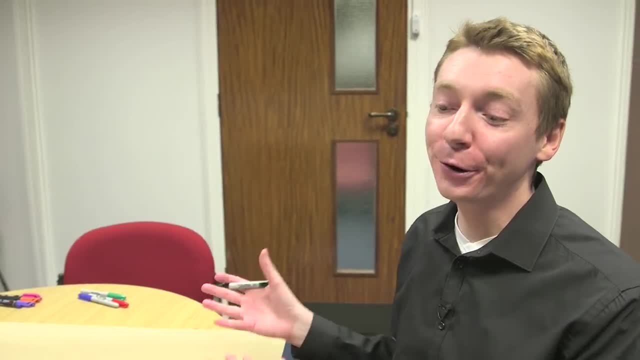 Euler's number, Would you have called it G? if you discovered it? I would not have called it G. No, I would have hoped somebody else would have called it G, and then I would have accepted that. Euler proved that this was irrational. He found a formula for E, which was a new formula. 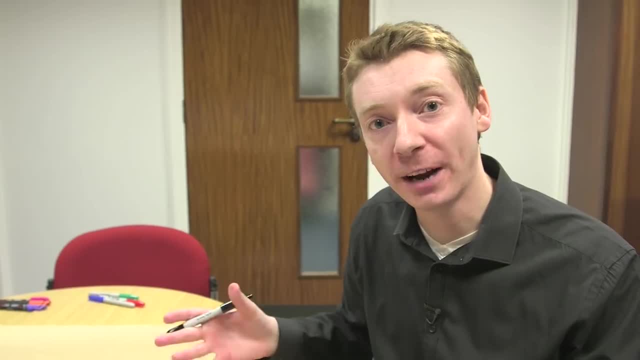 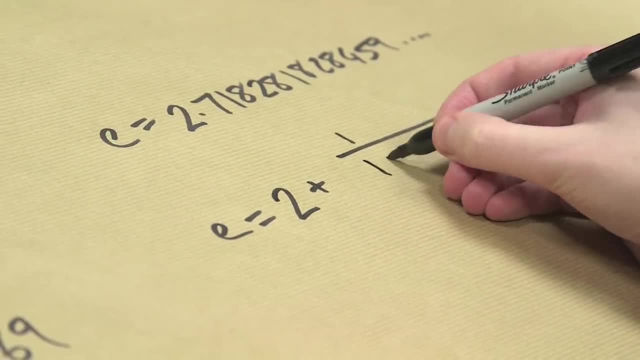 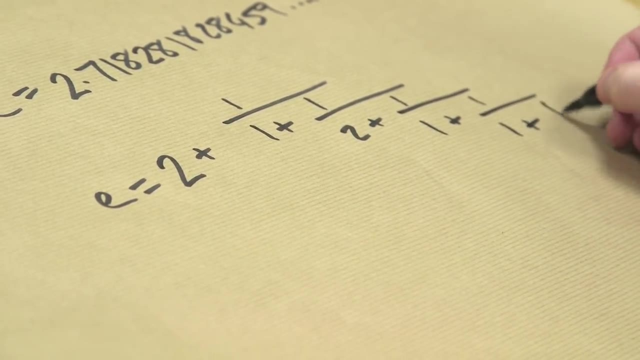 He found that E was equal to G, He found that E was equal to E, And that's the final place. And so it's T, And so it's O2, plus one over 11, plus one over two, plus one over one, plus one over one plus. 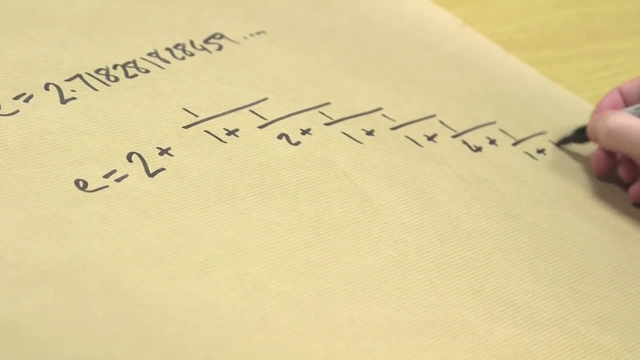 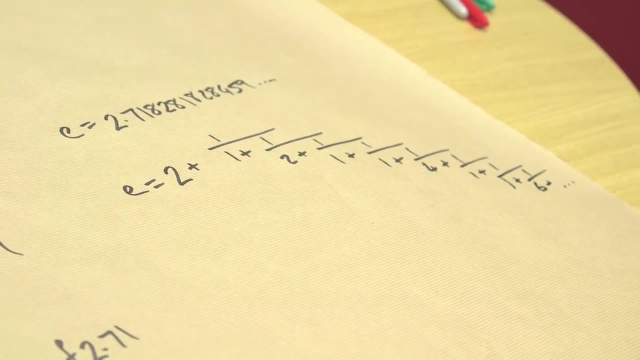 one over four, plus one over one, plus one over one, plus one over six, plus, And this goes on forever. This is a fraction that goes on forever, Continuous fraction, But you can see it goes on forever because there's a pattern and that pattern does hold. 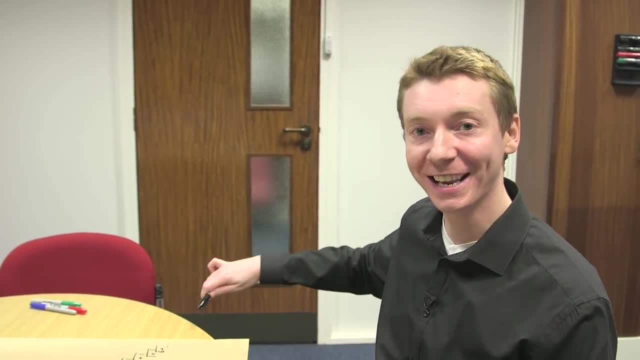 You've got two, one, one, four, one, one, two, 1, 1, 6, 1, 1, 8.. So you can see that pattern goes on forever. and if the fraction goes on forever, 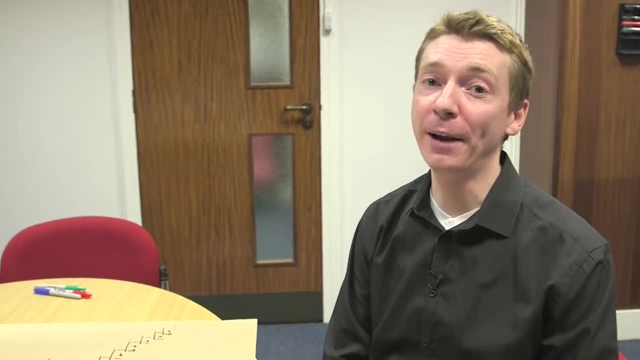 it means it's an irrational number. If it didn't go on forever it would terminate, and if it terminates you can write it as a fraction. And he also worked out the value for e. He did it up to 18 decimal places. 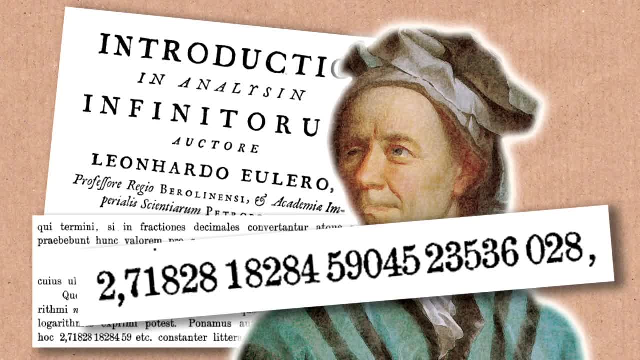 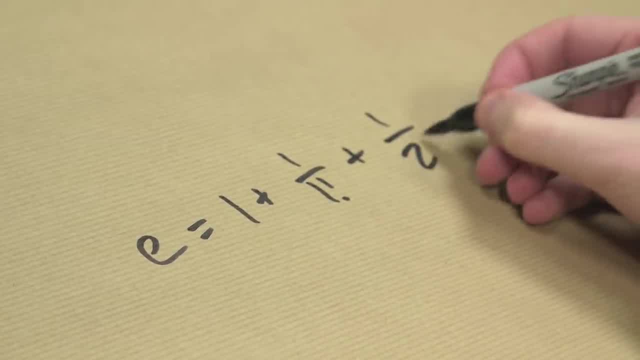 To do that. he had a different formula to do that. I'll show you that one. So this time he worked out: e was equal to 1 plus 1 over 1 factorial, plus 1 over 2 factorial plus 1 over 3 factorial plus 1 over 4 factorial. 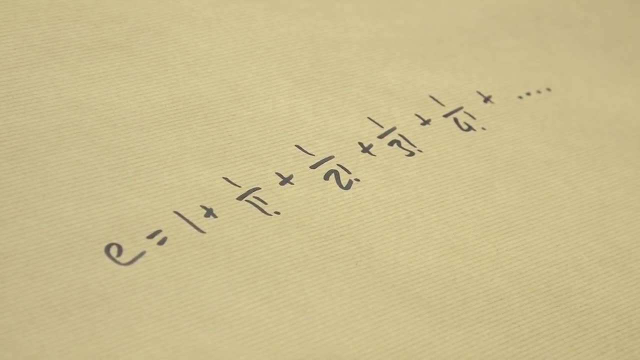 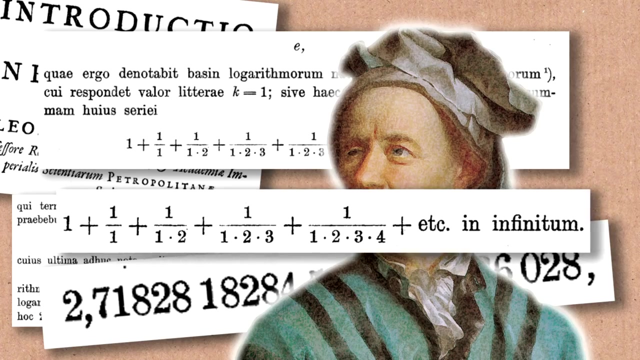 and this is something that's going on forever. It's a nice formula: If you're happy with factorials. factorials means you're multiplying all the numbers up to that value. So if it was 4 factorial, it'd be 4 times 3 times 2 times 1.. Okay, why is e a big deal? 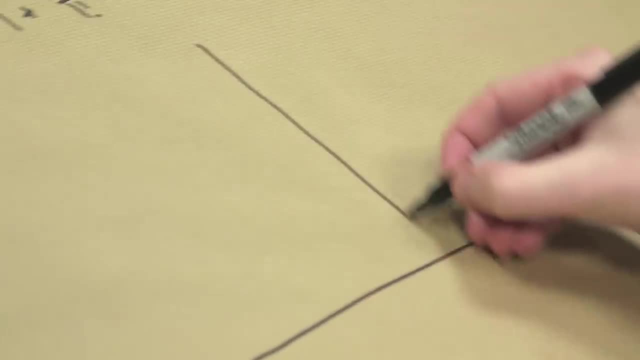 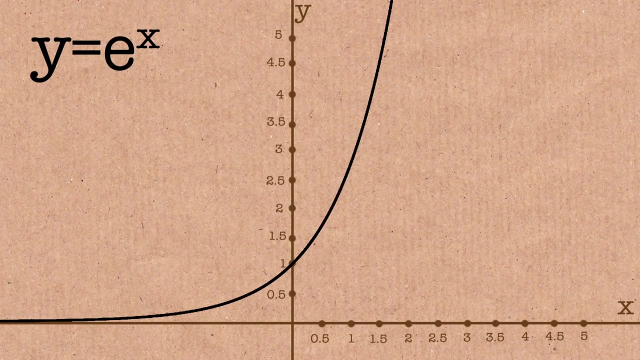 It's because e is the natural language of growth, and I'll show you why. Okay, let's draw a graph. y equals e to the x, So we're taking powers of e. So here, at 0,, this would cross at 1.. 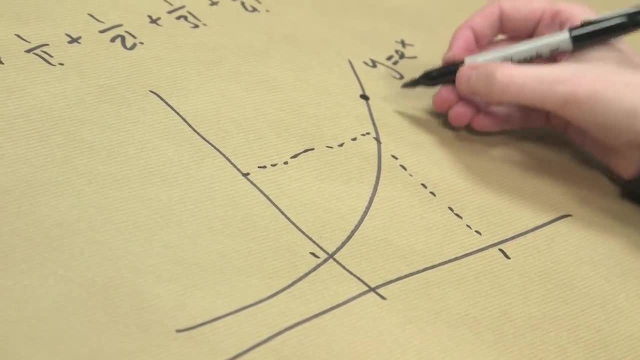 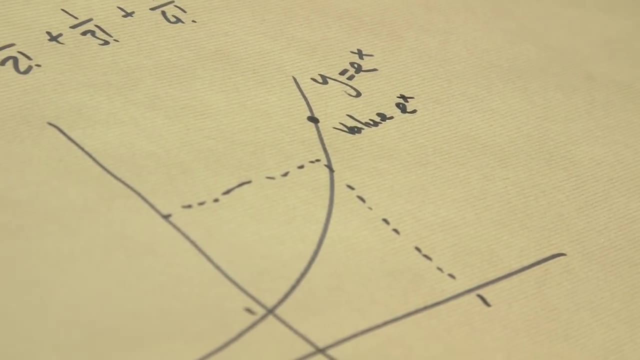 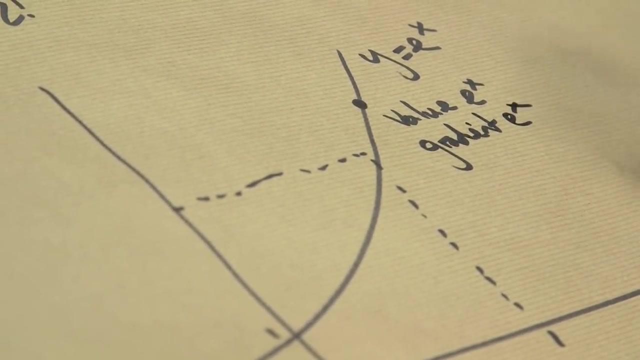 So if you took a point on this graph right, the value at that point is e to the power x And this is why it's important. The gradient at that point, the gradient of the curve at that point, is e to the x And the area 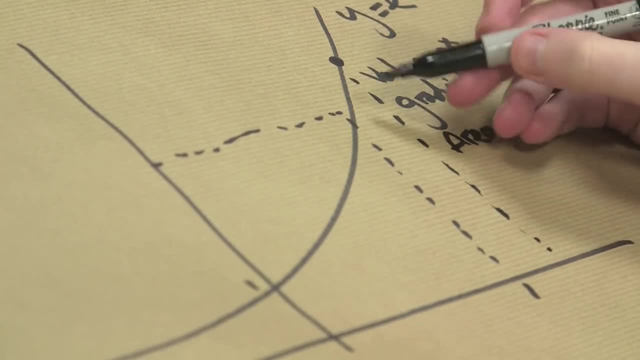 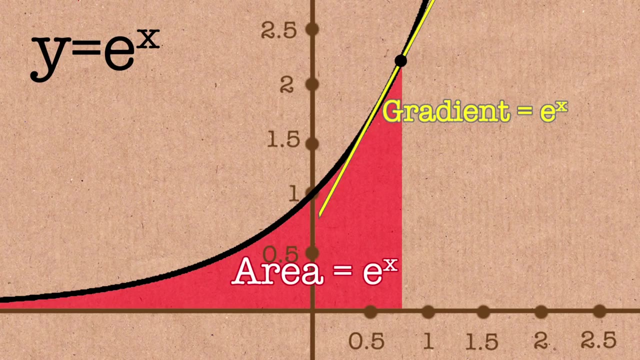 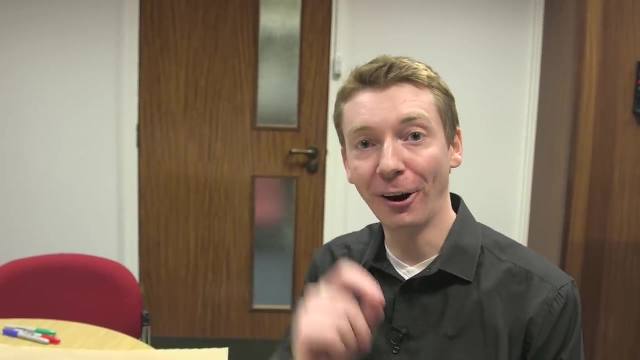 under the curve, which means the area under the curve all the way down to minus infinity, is e to the x, And it's the only function that has that property. So it has the same value, gradient and area- at every point along the line. 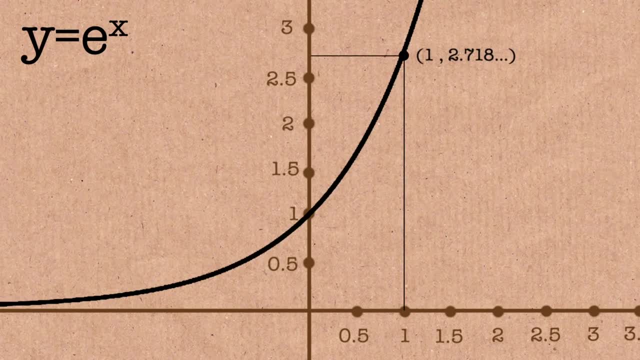 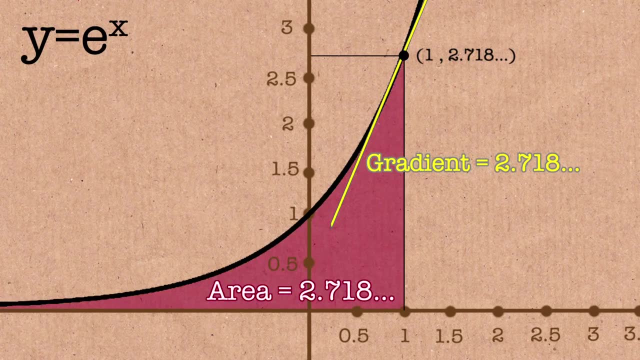 So, at 1, the value is e because it's e to the power 1.. The value is 2.718,, the gradient is 2.718, and the area under the curve is 2.718.. The reason this is important, then, because it's unique in having this property as well. 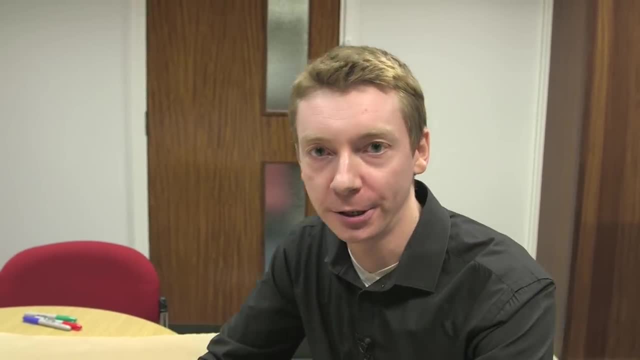 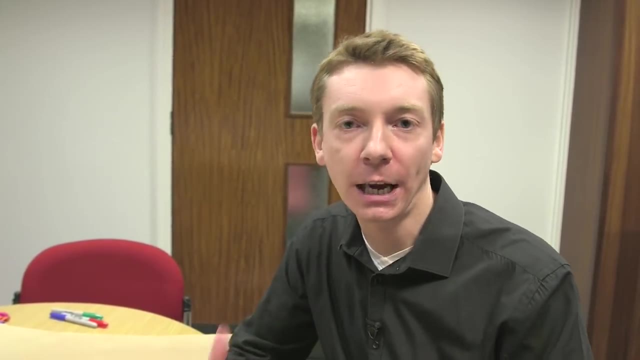 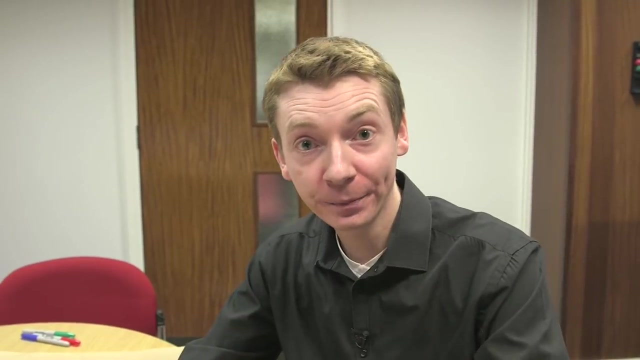 it becomes the natural language of calculus And calculus is the maths of rate of change and growth and areas, maths like that. And if you are interested in those things, if you write it in terms of e, then the maths becomes much simpler. Because if you don't write it in terms of e, you get lots of nasty constants and the maths is really messy. If you're trying to deliberately avoid using e, you're making it hard for yourself. It's the natural language of growth. 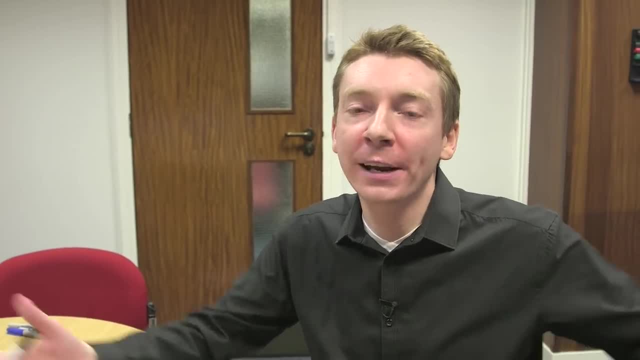 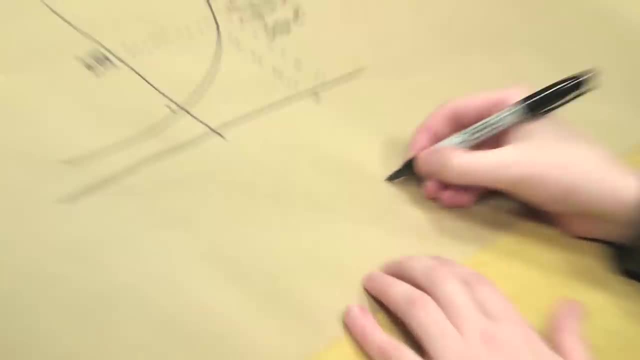 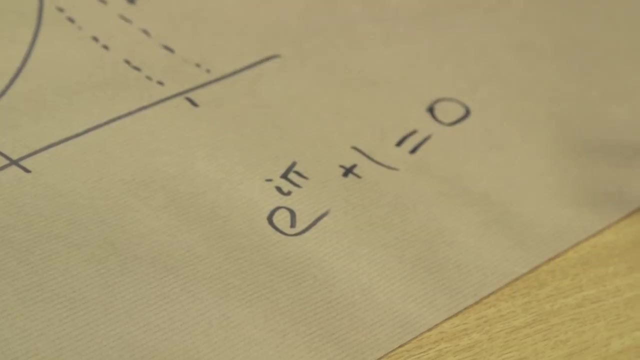 And of course, e is famous for bringing together all the famous mathematical constants. with this formula, Euler's formula, which is e to the i, pi plus 1, equals 0. So there we have all the big mathematical constants in one formula brought together. 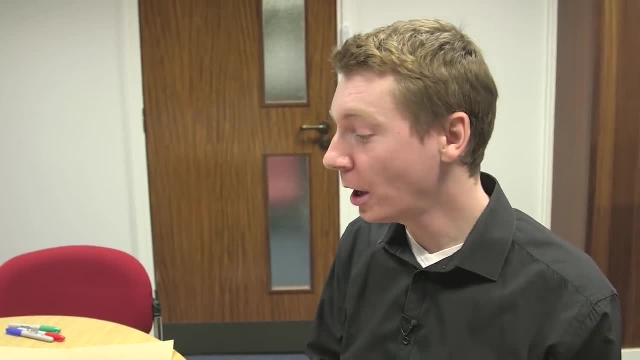 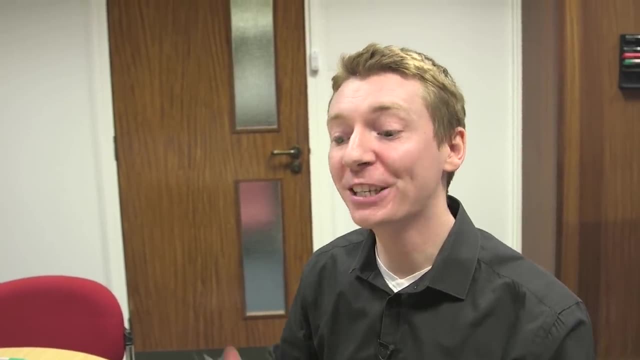 We've got e, we've got i, square root of minus 1, we've got pi, of course, we've got 1 and 0, and they bring them all together in one formula, which is often voted as the most beautiful formula in mathematics. 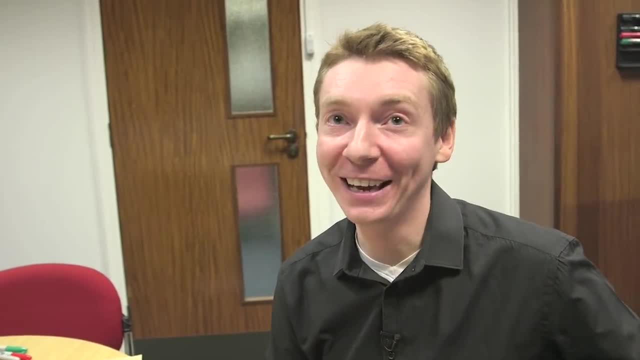 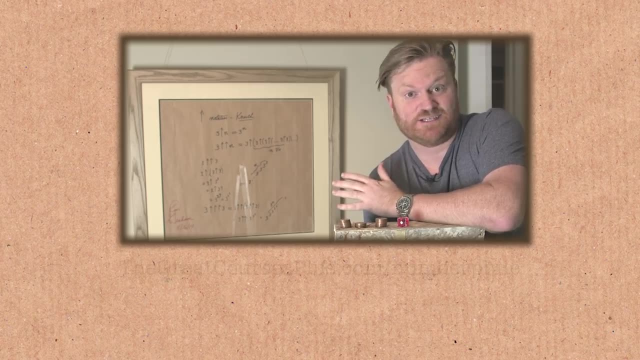 I've seen it so often that I'm kind of jaded to it. Don't put that in the video. Sometimes here on Numberphile we can make more videos than we'd otherwise be able to thanks to excellent sponsors, And today we'd like to thank The Great Courses Plus, which is a fabulous service. 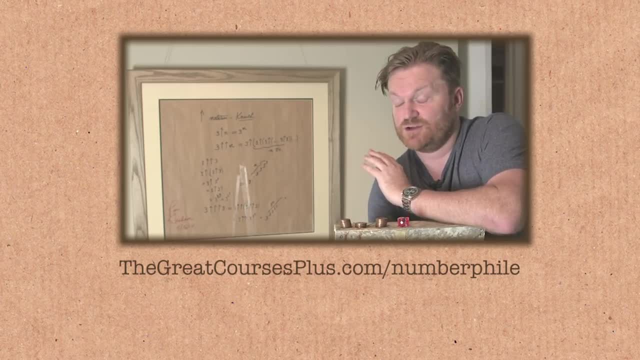 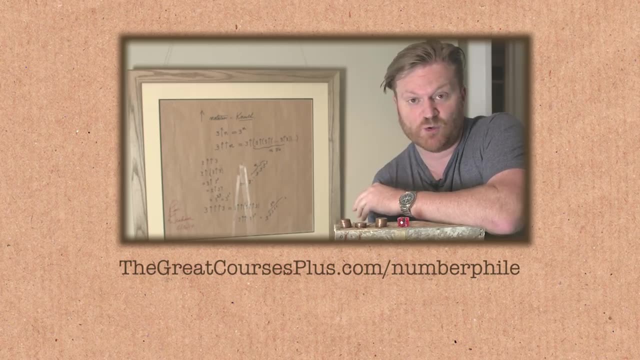 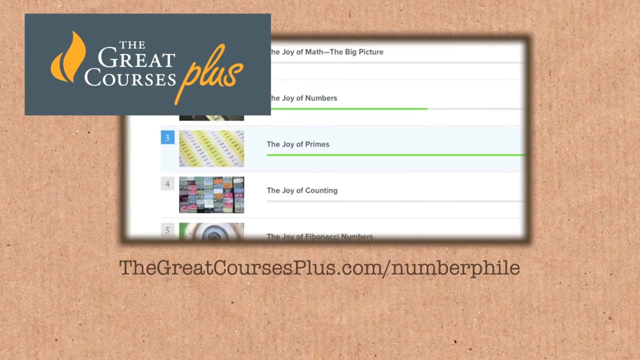 If you like Numberphile videos, you're really going to like this. They've got an incredible array of lessons- something like over 7,000 videos from world experts, top professors around the world on all sorts of subjects, from photography to paleontology to prime numbers. No matter what you're into, you're going to find something. 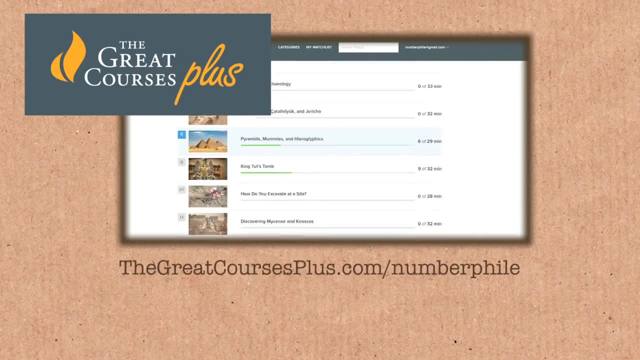 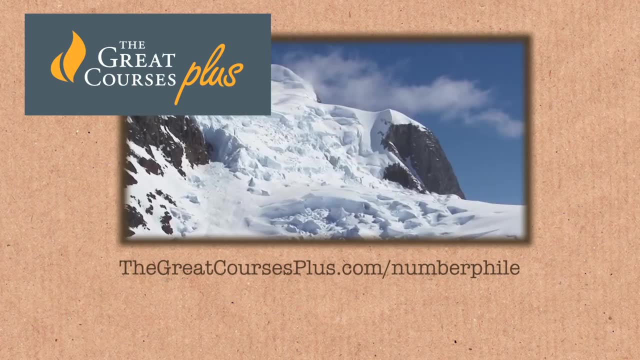 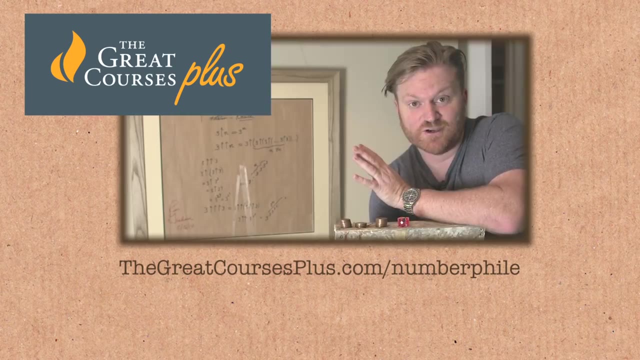 What I've been looking at just recently on the site is paleontology and one of my favorite subjects, Egyptology. They've got some great videos on those. Now, plans on The Great Courses Plus start from $14.99 a month, but there's a special offer where you can go and get a whole month unlimited access to all the videos for free.